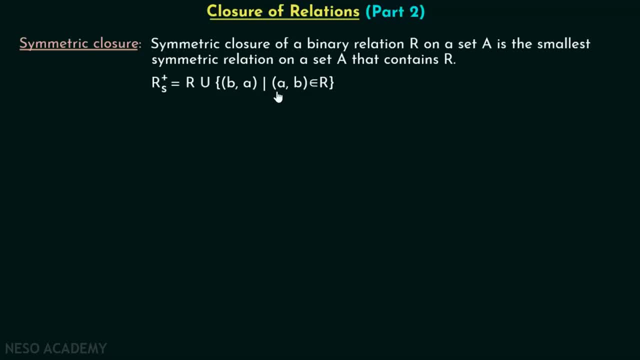 such that A- B belong to R. If A B is there in R, then B A must be included in R, S plus. It is as simple as that. So here is one problem related to symmetric closure. Let R be the relation on the set 0,, 1,, 2,, 3. 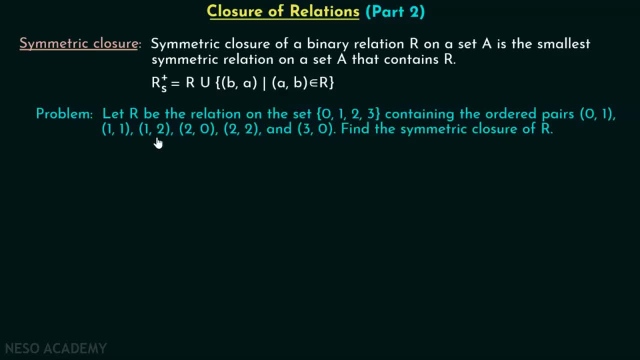 containing the ordered pairs 0, 1, 1, 1, 1, 2, 2, 0, 2, 2 and 3, 0.. Find the symmetric closure of R. We are interested in finding the symmetric closure of relation R. 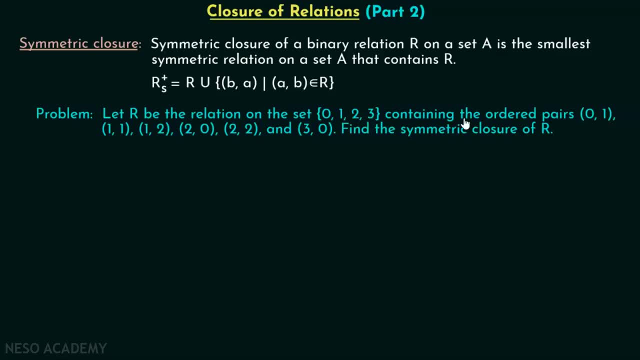 which is defined on the set 0, 1, 2, 3, and it consists of these ordered pairs: 0, 1, 1, 1, 1, 2, 2, 0, 2, 2 and 3, 0. 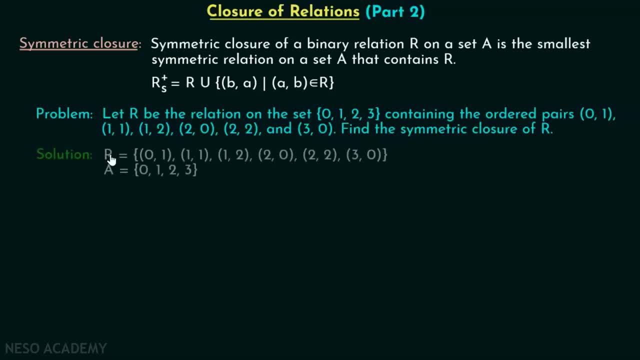 Okay, Let's find out the solution Here. you can see, this is our relation, which consists of these ordered pairs, and we have set A, which consists of these elements. Okay, Again, this is just a letter I have chosen for this particular set. 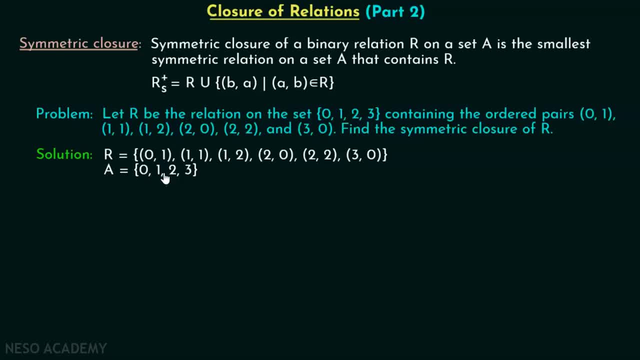 It is up to you that which letter you want to choose for this set Doesn't matter. I just want to name this set. Okay, Now we are interested in finding the symmetric closure of R. What is symmetric closure of R? R S plus is nothing but equal to. 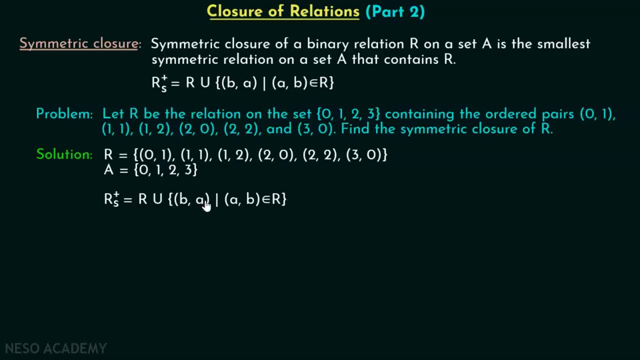 R union with set of all ordered pairs B, A, such that A B belong to R Right First. we must include R in R S plus. That means we must include all the ordered pairs of R inside R S plus. So 0, 1, 1, 1, 1, 2, 2, 0, 2, 2, 3, 0 must be there in R S plus. 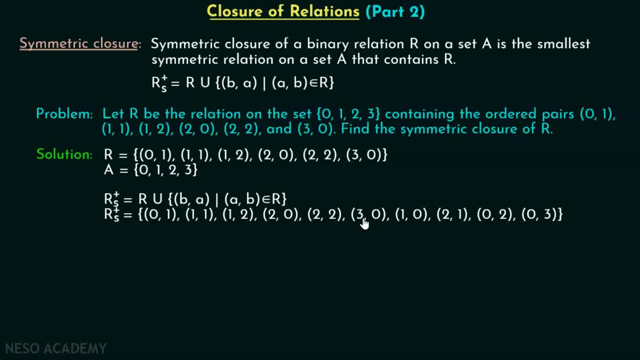 As you can see that 0,, 1,, 1,, 1,, 1,, 2,, 2,, 0,, 2,, 2,, 3,, 0 is there in R S plus. Apart from this, for every A, B belong to R. 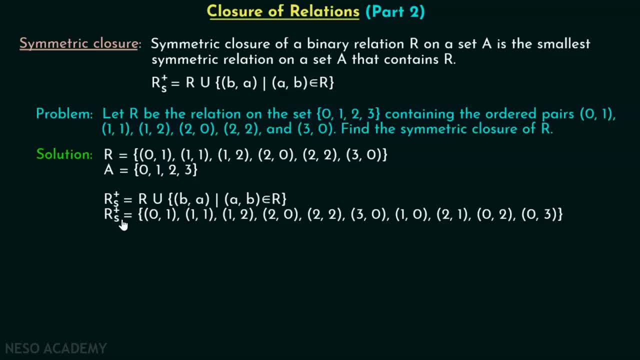 we must include B A in this R S plus. Then only we can say: it becomes symmetric relation, Right? We can see that 0, 1, 1, 2, 2, 2, 3, 0, 2, 3, 0 is there in R S plus. 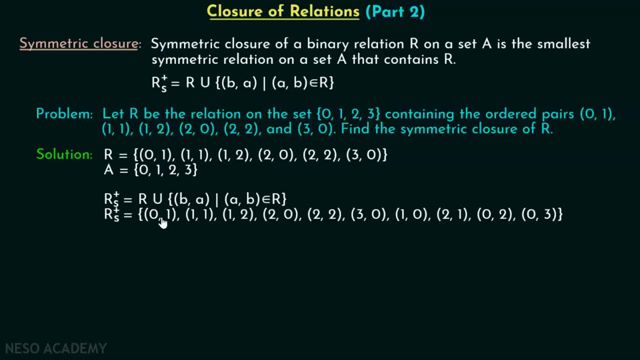 We can see that 0, 1,, 1, 1, 2,, 2,, 2,, 2,, 3, 0 is there in R S plus, But there is no 1, 0 in this relation. 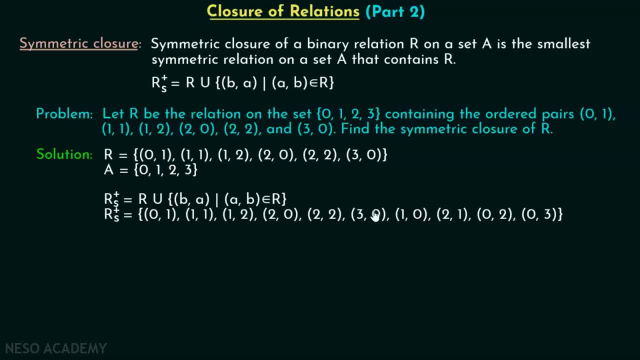 Right. Therefore, 1, 0 must be included. Apart from this, we have 1, 2,, but there is no 2, 1.. So 2, 1 must be included. We can see that 2, 0 is there in this R S plus. 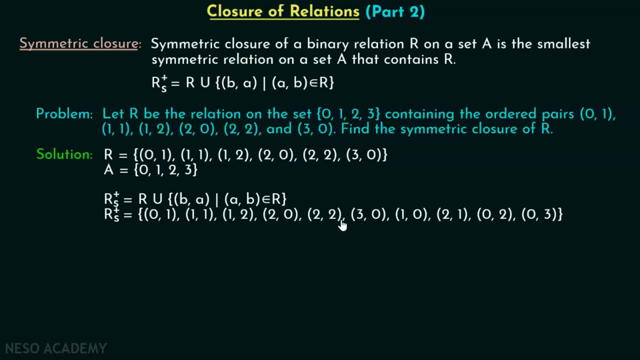 but there is no 0, 2.. So 0, 2 must be included. Apart from this, we have 3, 0.. So 0, 3 must be included. Now it is complete. This R S plus is now complete. 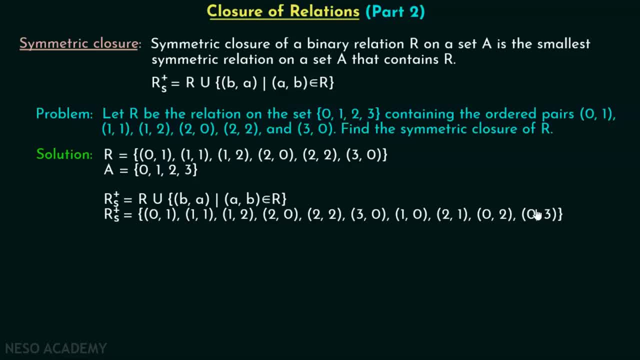 And now you can see that this is a symmetric relation, And let me tell you, this is the smallest symmetric relation possible, which contains R. Right, Let me reorder this once again, So this becomes 0, 1, 0, 2, 0, 3, 1, 0, 1, 1, 1, 2, 2, 0, 2, 1, 2, 2, 3, 0.. 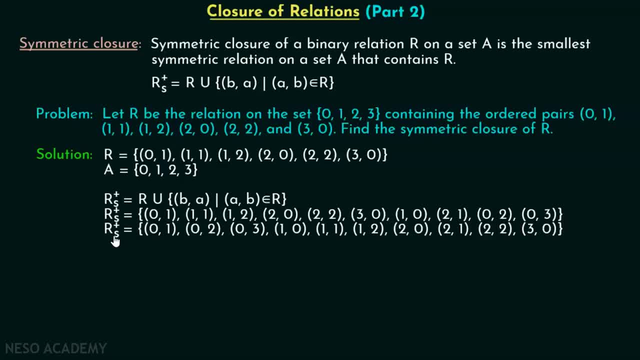 These are all the ordered pairs of R, S plus. This is the smallest symmetric relation on a set A that contains R. Okay, That's it. This is all about symmetric closure. Now we will discuss what is transitive closure. Okay, 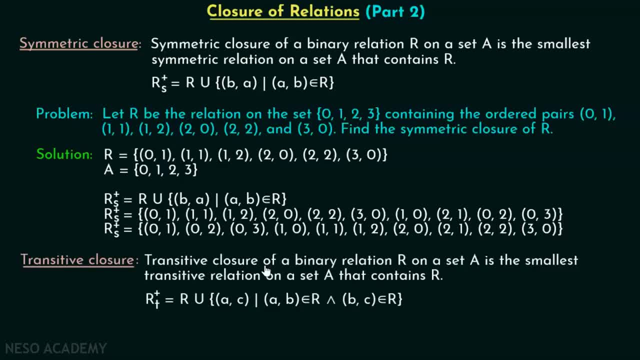 Transitive closure of a relation R on a set A is the smallest transitive relation on a set A that contains R. Quite obvious, right. Symmetric closure of a binary relation R on a set A is the smallest symmetric relation on a set A that contains R. 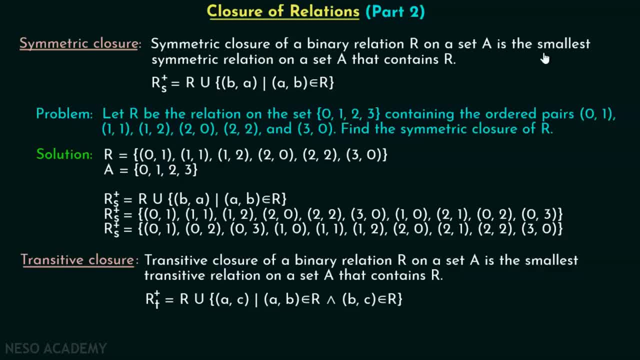 Right. We know that in case of symmetric closure, we are considering the smallest symmetric relation. Here we must consider smallest transitive relation, Right. So transitive closure of a binary relation, R on a set A, is a small. In this case we are considering the smallest transitive relation on a set A that contains R. 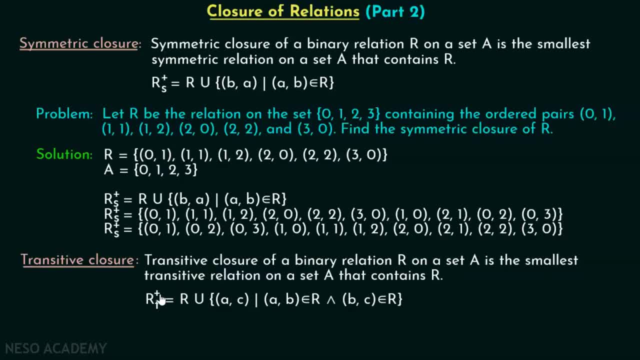 Transitive closure of a binary relation. R is denoted by R T plus, and this must be equal to R union with set of all ordered pairs A- C, such that A- B belong to R and B C belong to R. This is important. 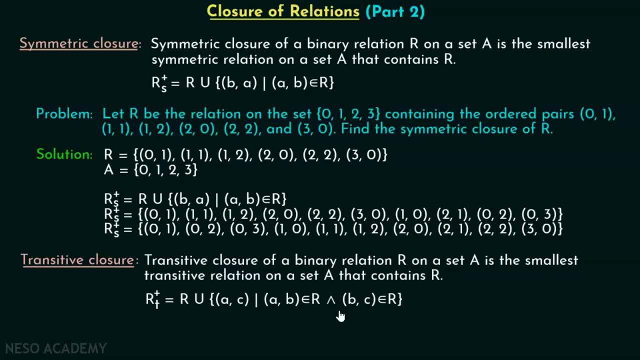 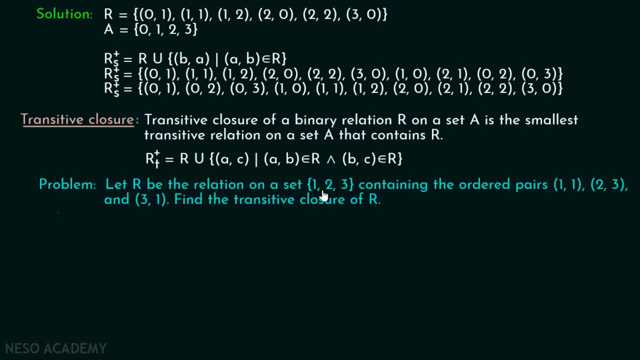 If AB belong to R and BC belong to R, then AC must be included in R in order to make that particular relation transitive, Isn't that so Now let's just start. So let's start. consider one problem related to transitive closure. Let r be the relation on a set: 1, 2, 3. 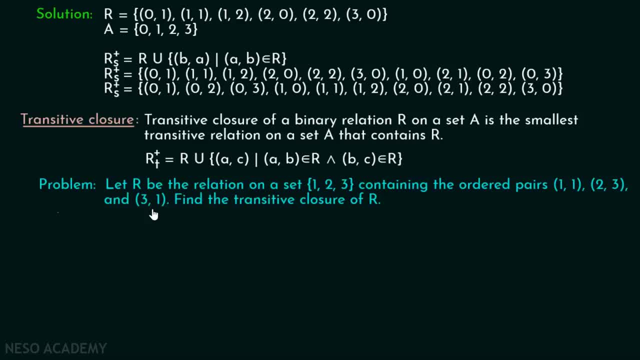 containing the ordered pairs 1,, 1,, 2,, 3 and 3, 1.. Find the transitive closure of r. We are interested in finding the transitive closure of this relation, r, which is defined on set 1,, 2, 3.. Okay, so we have.